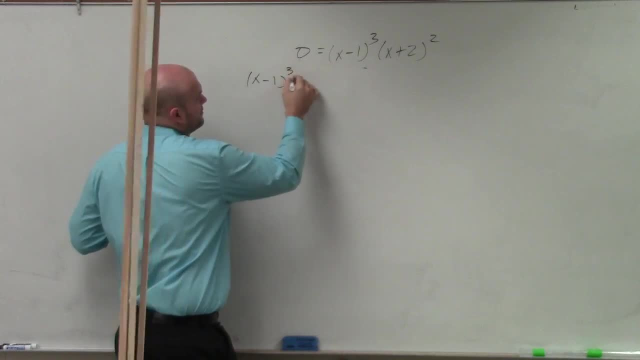 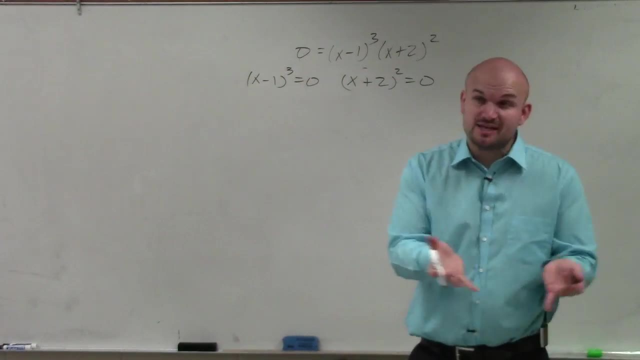 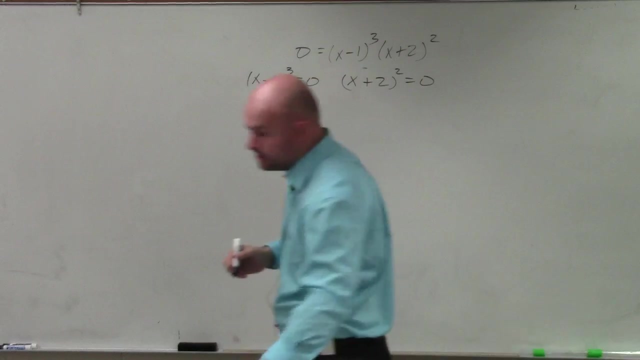 Now I can apply my 0 product property. However, before I can do anything inside the parentheses, I have to undo what's happening outside the parentheses, which looks like cubing and squaring. So I need to undo the cube root or undo cubing. 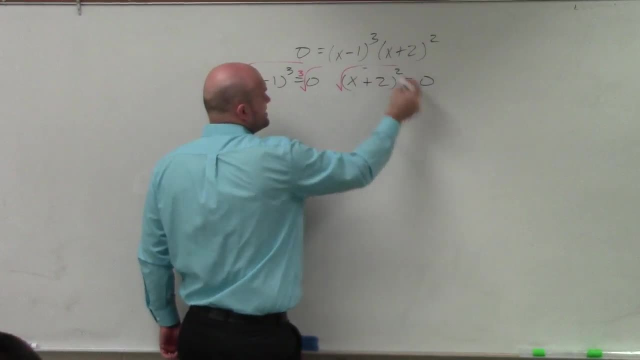 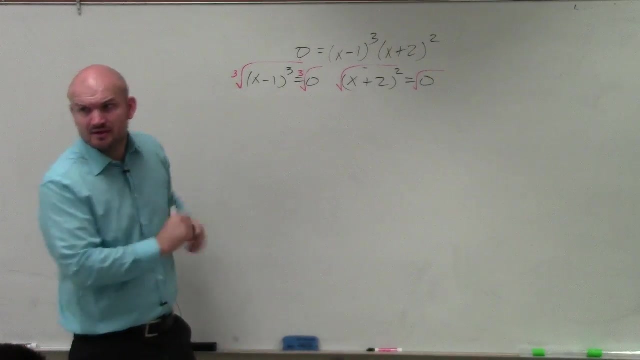 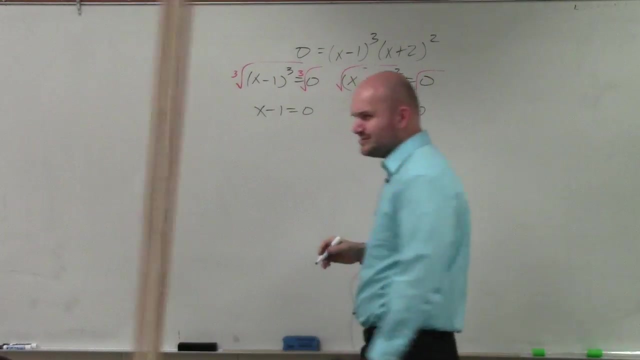 by taking the cube root of both sides Undo the square root. by taking the square root of both sides. Notice guys, it doesn't really matter what power my factor is raised to, I'm still going to have whatever's inside the parentheses equal to 0.. 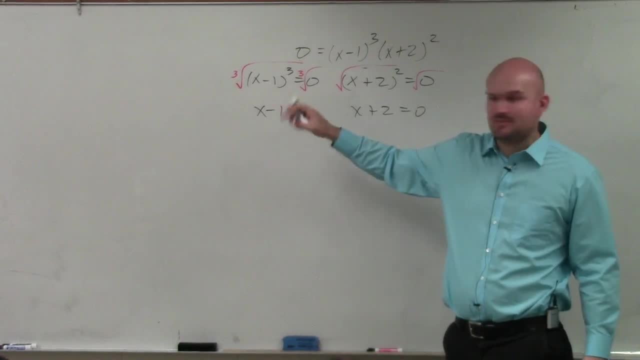 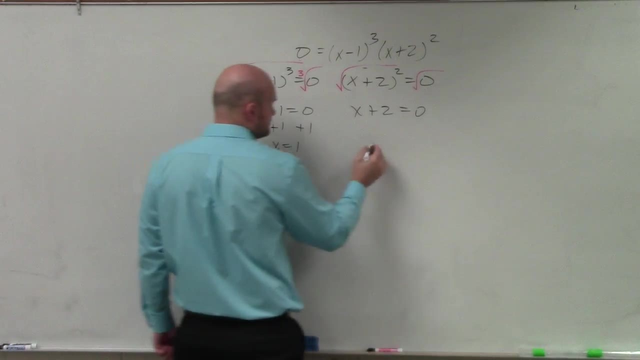 So it doesn't matter if I raise it to the 18th power or the 15th power. Whatever's inside my parentheses is still going to be my 0. Now I just add 1, add 1.. So x equals 1.. 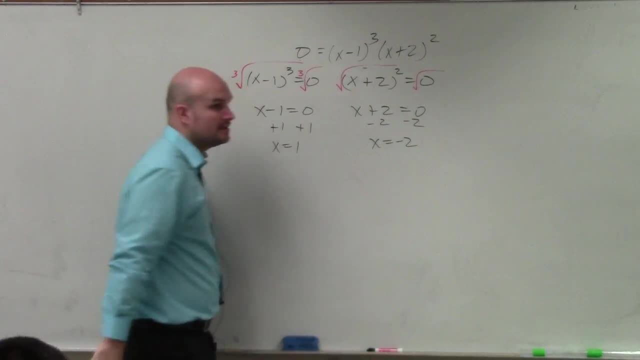 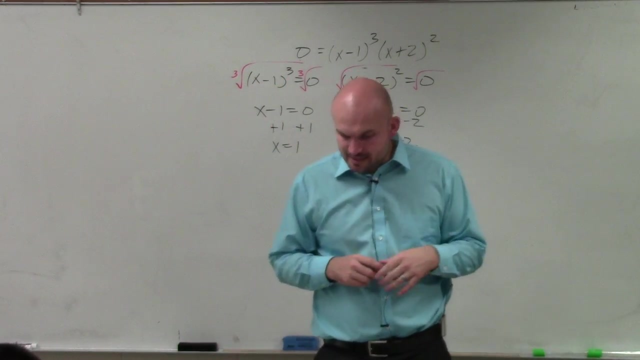 Subtract 2, subtract 2.. x equals negative 2.. Those are my 0s. However, it asks us now to identify the multiplicity and state: does the graph cross or does it bounce? So, when identifying multiplicity, what we're looking at is we're looking. 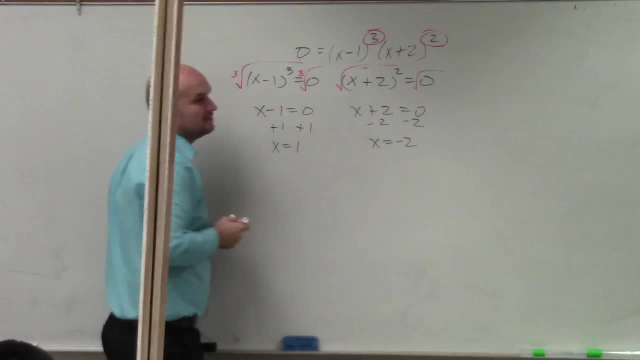 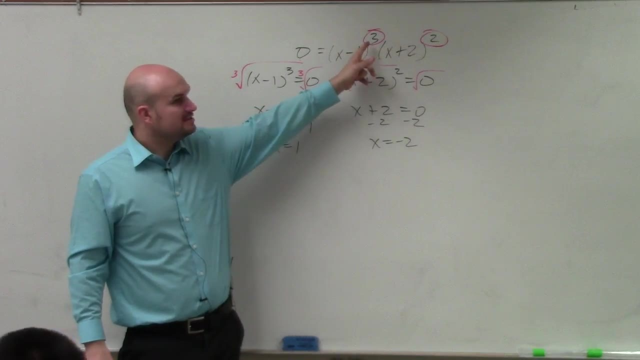 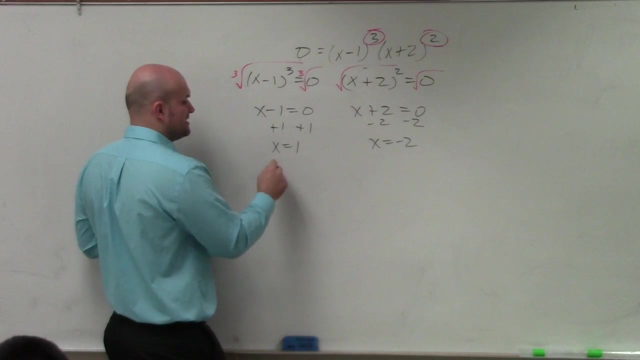 at the power of the factor. So, while that 3, please be very careful- while that 3 does not affect this value of the 0,, it does affect the graph And that is what we call our multiplicity, where we can say the multiplicity of my 0 at x. 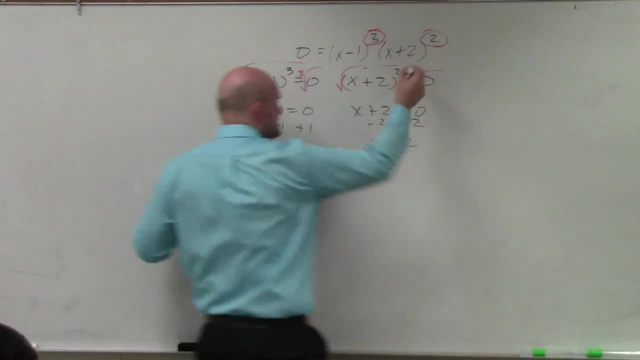 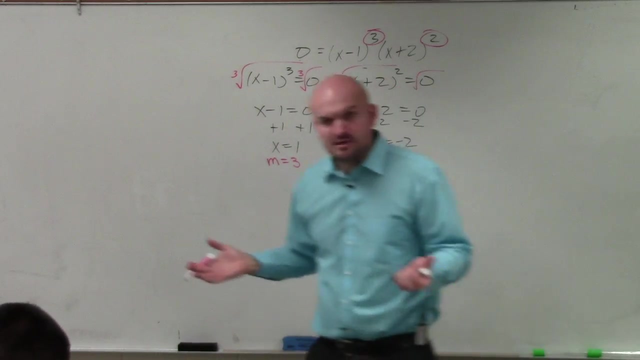 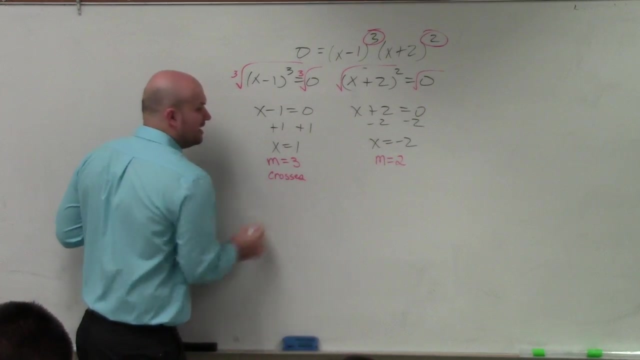 equals 1 is equal to 3.. The multiplicity of my 0 x equals negative 2 is equal to 2.. 2. Now why again is multiplicity important? Because if the multiplicity of a 0 is odd, it crosses. 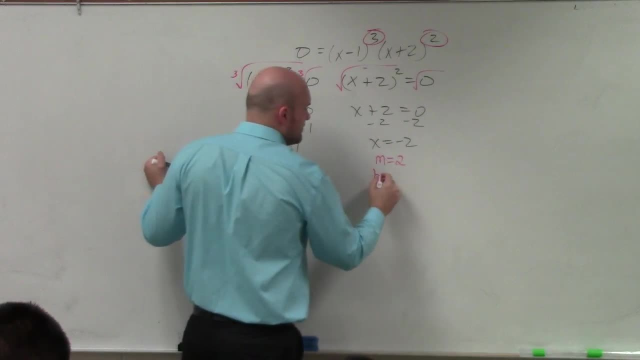 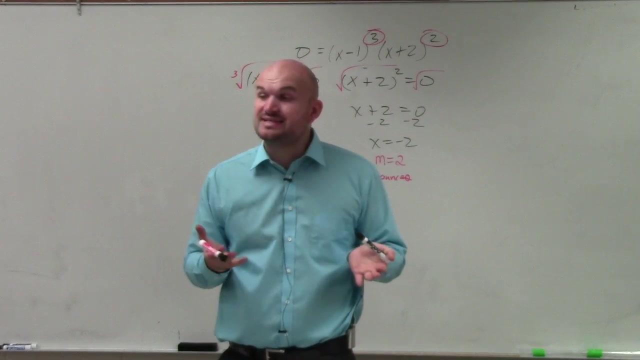 If the multiplicity at a 0 is even, it bounces. Now to sketch this. they asked us to sketch this by hand. You could use graphing technology and I would have no problem with that. But I'm just going to show you real quick. 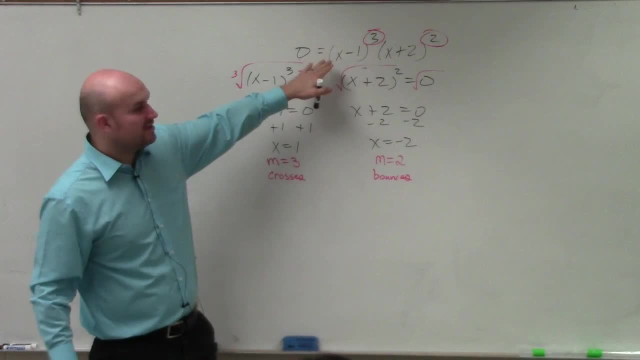 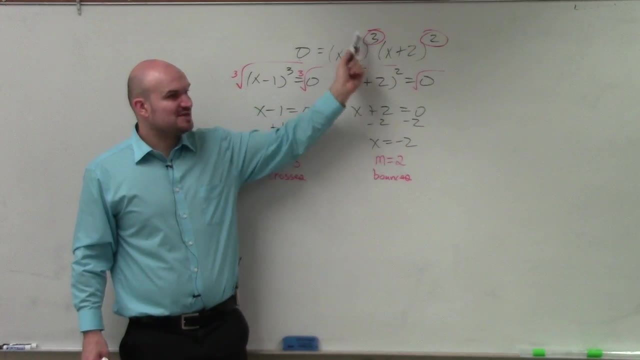 because this will help you out for your quiz as well. Can we identify What the end behavior would be of this polynomial? Yes, Let's try to find the degree. If I did x minus 1 cubed, what would be the degree of that? 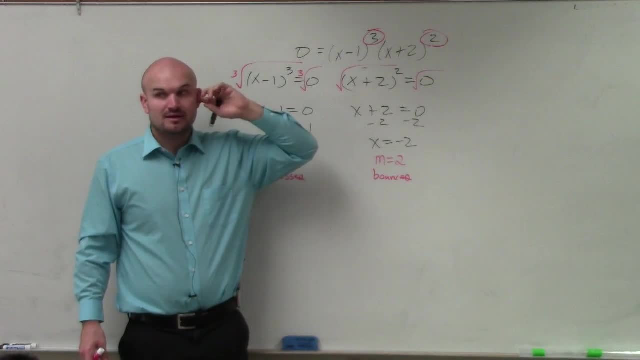 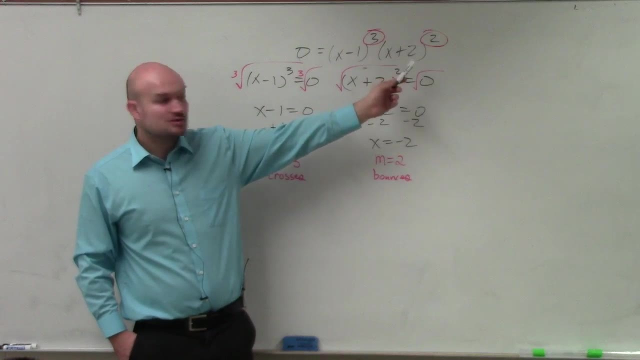 If I were to expand that out, the highest power would be x to the third power, which would be x cubed. And if I was to expand x plus 2 squared, that would give me x squared. So I'd have an x squared times an x cubed, which.